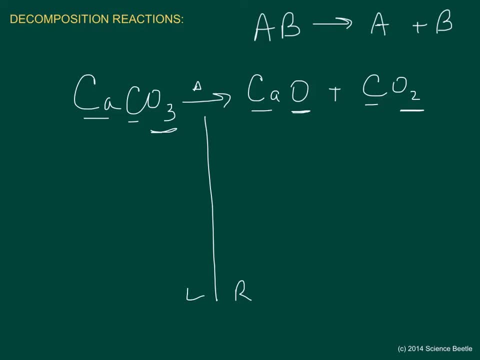 But we've got two oxygens bound to carbon. That gives us a total of three. So, right off the bat, what we notice is that we have an equation here that is completely balanced. So there's really not much for us to do except here is to go ahead and to count our various parts. 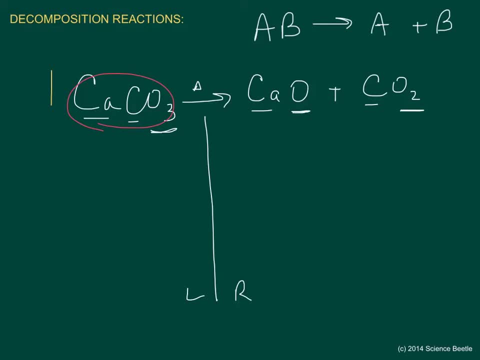 And so here we've got one compound, So that will give us a coefficient of a one. And on the right-hand side we've got one calcium oxide, So that will give us a coefficient of one. And we've got one carbon dioxide, which will also give us a coefficient of one. 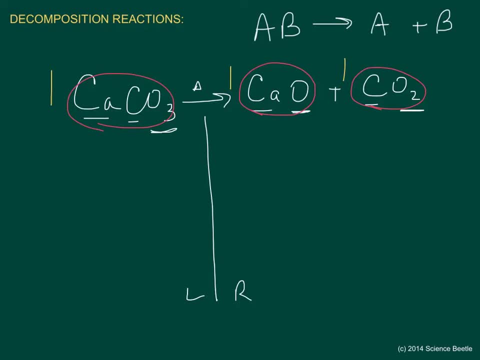 If this was a multiple choice test or multiple choice quiz. what you want to do is you want to go ahead and find the answer or the choice, either from whatever amount of options you've got. Look for the choice that gives you the following: 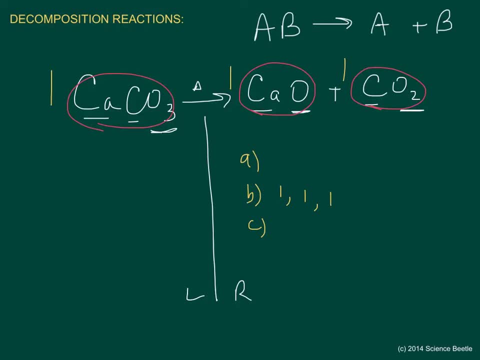 One comma, one comma one, And looking at from previous videos, this first one relates to the first mole number or the first coefficient, The second one relates to the second coefficient And the third one relates to the third coefficient in this sample problem. 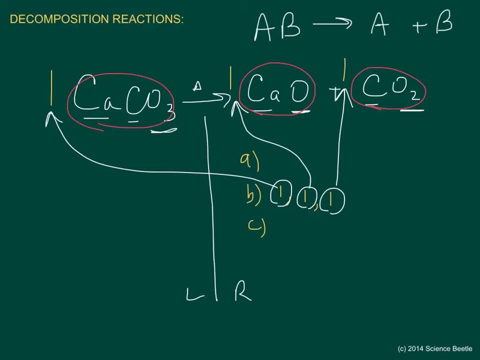 Now, this one was pretty easy for us to do, But let's go ahead and look at a little bit more complicated one that is going to require us to do a little bit more balancing. So, for this problem, what we're going to do is we're going to take this equation here that we've got. 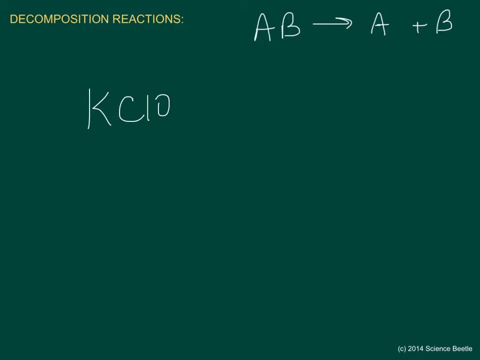 We're going to take KClO Three And we're going to go ahead and react this or apply this to a substance which is what we call KCl. That's what we're going to get, Plus oxygen. Now we are mixing this in a solution of manganese oxide. 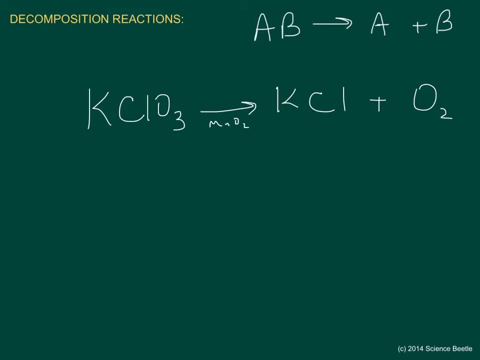 which is MnO2 with a little bit of heat, And that's what that represents there, But essentially, what we're paying attention to is the KClO3 on the left-hand side. Okay, here's the left, here's the right. 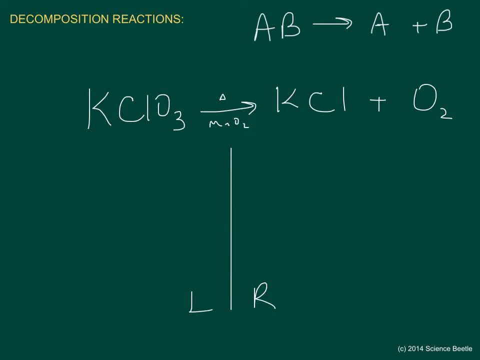 And we're going to see the products KCl and oxygen on the right, And what our goal today is just to simply balance it. So we'll begin with the first atom, and that's going to be the calcium on the left-hand side. 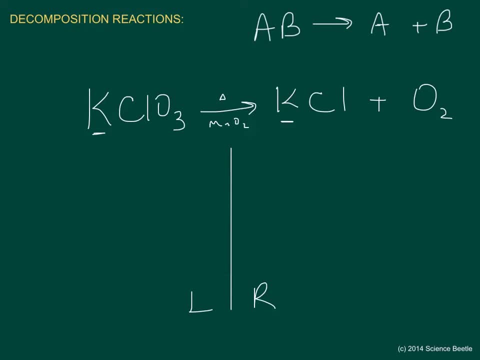 So we look on the right-hand side and we notice that we have one calcium. So our calciums are balanced because we have the same number on the left as we do on the right. We then move on to our chlorines. 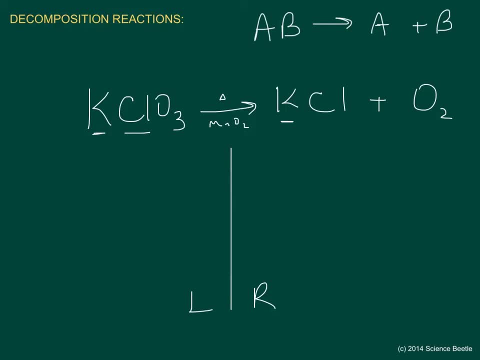 We've got one chlorine on the left, And we look at the calcium, We look on the right-hand side and we notice that we've got one chlorine as well. So so far so good. Everything is balanced. We've got the same number of potassiums. 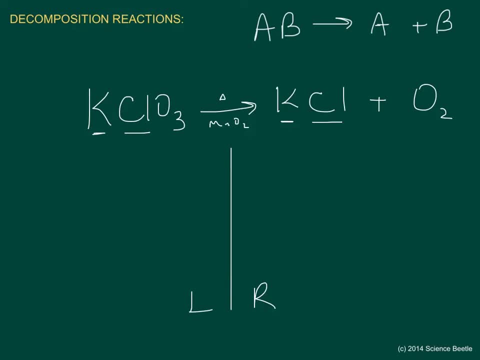 We've got the same number of chlorines. We now turn our attention to the oxygens And, if you notice, on the left-hand side you've got three oxygens on the left And on the right-hand side you've got two. 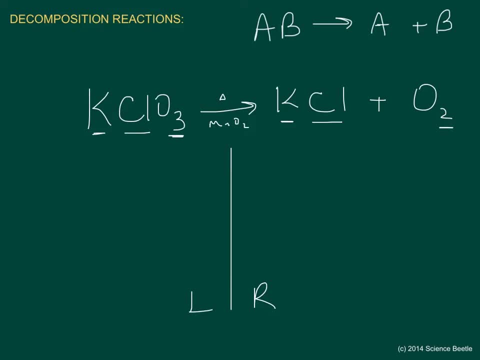 Now, at this point, what we want to do is we want to focus on this three And we want to make sure that we can convert this into an even number. The easiest way for us to do that is to add another whole compound of KClO3.. 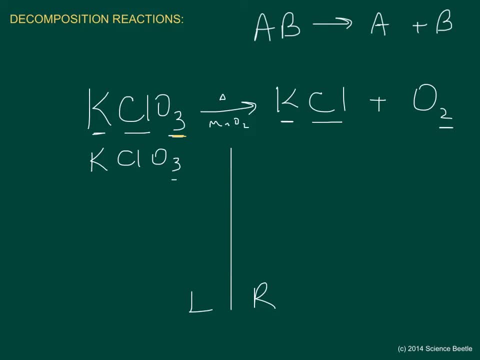 Now, if we look at the oxygens at this point, you're going to notice that we've got a total of six, Which means that on the oxygens on the right-hand side, we need to add another oxygen molecule. excuse me, 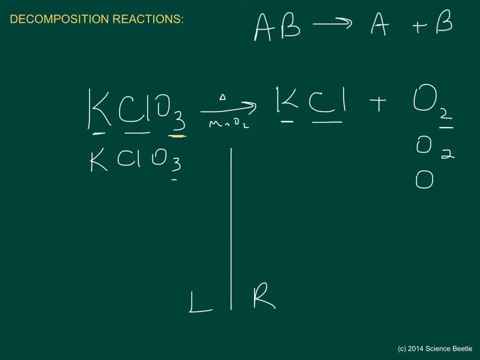 and another oxycon, oxygen molecule- Pardon me again- For a total of six oxygens here on the right-hand side. Okay, so we can see that here There's one, two, four and six. 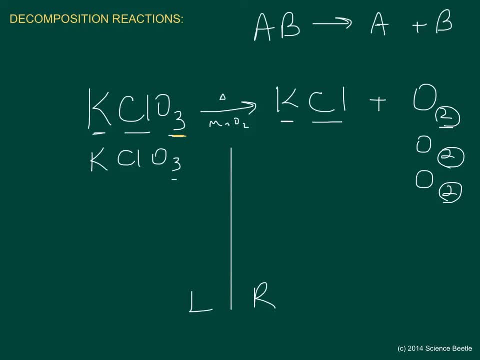 So we've got six oxygens on the right-hand side, We've got six oxygens on the left-hand side, And so now we turn our attention to the potassiums at the very beginning, Because we notice, when we added that potassium, KClO3 on the left-hand side, what happened is we added another chlorine and we added another potassium. 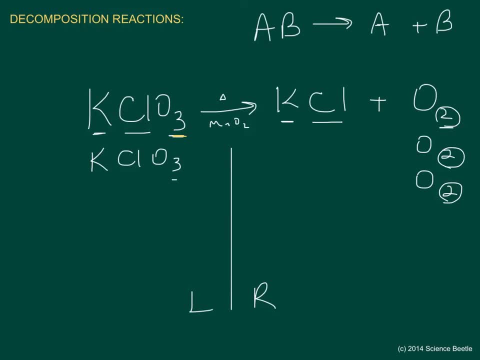 So we'll go ahead and address this right away. We've got two potassiums on the left-hand side, which means we're going to have to add another potassium and a chlorine compound, And by doing that we also solve the problem that we have with our chlorine. 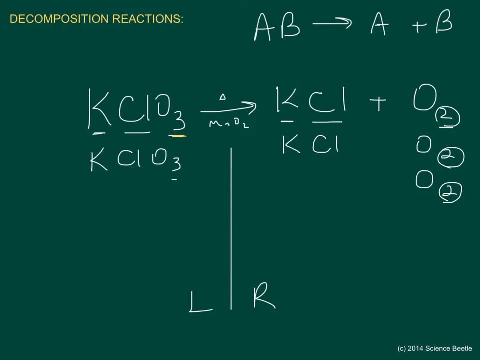 So we have two chlorines on the left as well as two chlorines on the right, And we have two potassiums on the left as well as two potassiums on the right. So now our reaction here is completely balanced. 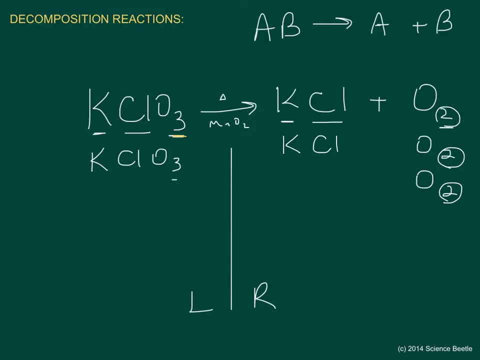 And all we have to do now is add up all the different compounds that we've got, or the different molecules. So here's one- two. So that means our coefficient for this section is going to be two. We go to the right-hand side and we've got one two.